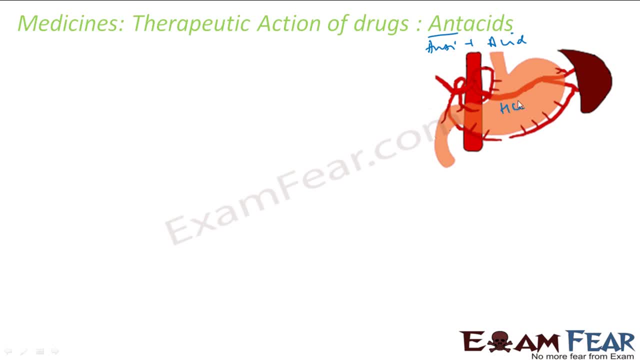 HCL and pepsin. sometimes the stomach overproduces the anti-acids and sometimes the stomach overproduces the anti-acids, anti-acids, anti-acids, HCL and pepsin. so this causes pain, it causes irritation and sometimes it is very serious, it may cause ulcer, correct? so what is the problem? statement: stomach. 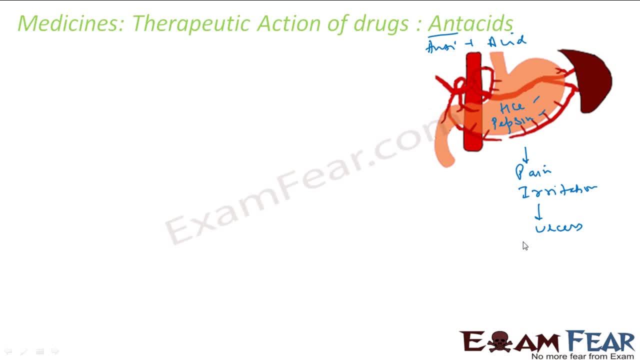 generally to digest the food. it creates hydrochloric acid and pepsi to digest food but sometimes the hydrochloric acid in the pepsin is too much in the stomach. it creates more and more hydrochloric acid and pepsi and that will cause you pain and irritation. it will also cause 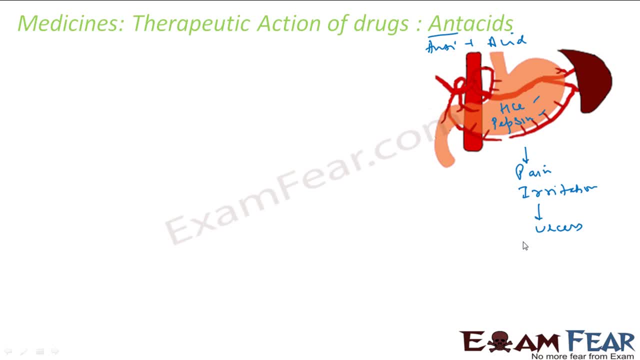 ulcer. if severe this scenario is called acidity in the stomach, it's called acidity in the stuff. you must have heard of the term acidity in the stuff. so to remove this, we need something which can take care of this acidity. so to remove this, we need something which can take care of this acidity. 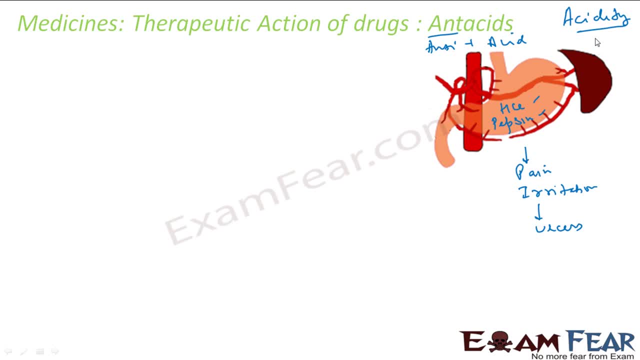 right. one option is: you can use the best. so in till 1970s, when not much treatment was there, the only treatment of this acidity was to use base. and they use na a co3, it is sodium hydrogen carbonate. to this sodium sodium hydrogen carbon is actually when it reacts with water in the body. 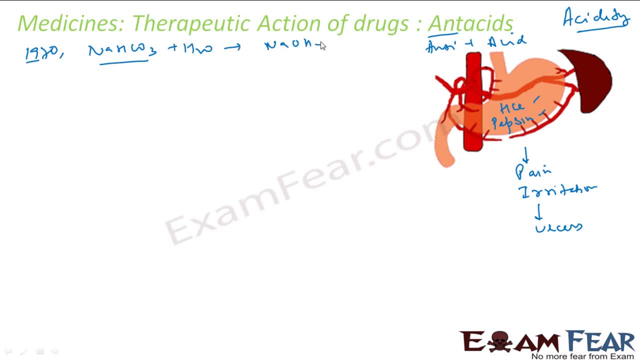 it used to produce any away water and carbon dioxide, as NOH is nothing but basic. so this basic, this base NOH will react with HCL to form NaCl and water correct. so this will make the whole stomach basic and the patient will feel. but there is a problem to this. the problem is if you use more NaCO3 sometimes. 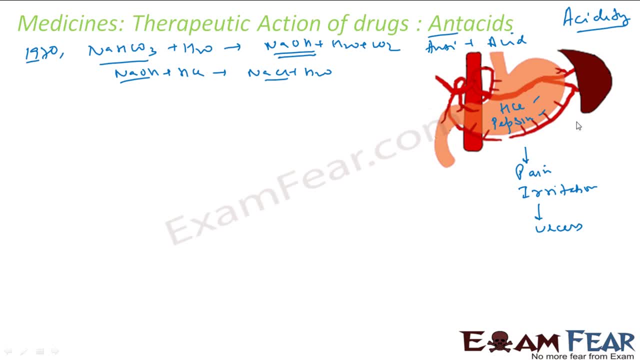 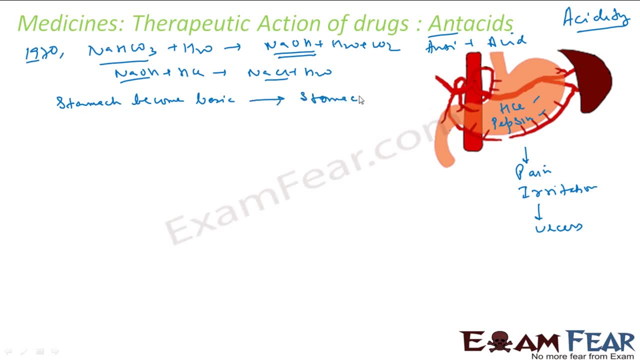 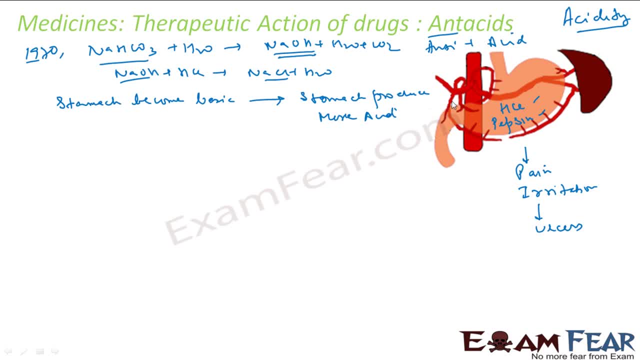 stomach produce more acid and in that case the whole acidity becomes worse. right, the patient gets more pain. so the next solution was, instead of nas co3 to use aluminum hydroxide and magnesium hydroxide mixture. all these correct, so these are better. they are better alternative. 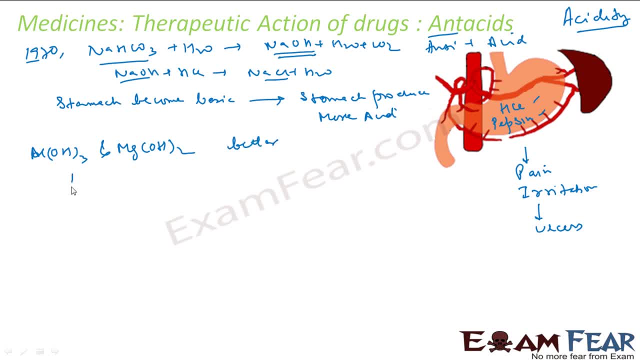 why? because they are insoluble. they are insoluble in water and it won't increase. increase the pH above neutrality at the max. it will make stomach neutral. it will not make more than neutral. so with that it is little better. but there is a problem with this. the 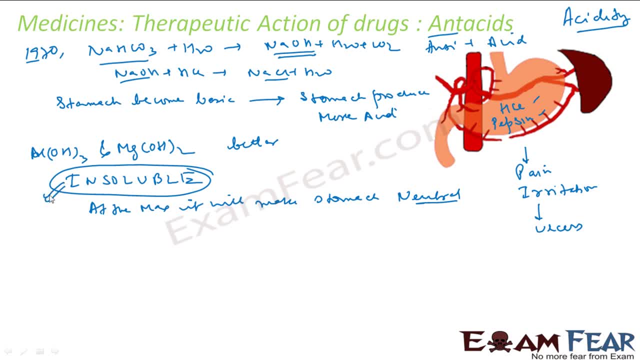 problem is this: they are insoluble, so they won't break down, so they will be in the body itself. it is not good to have so many insoluble compounds in the body, undesirable, correct. so nothing is foolproof now and it has to be controlled because this acidity, if it is not,